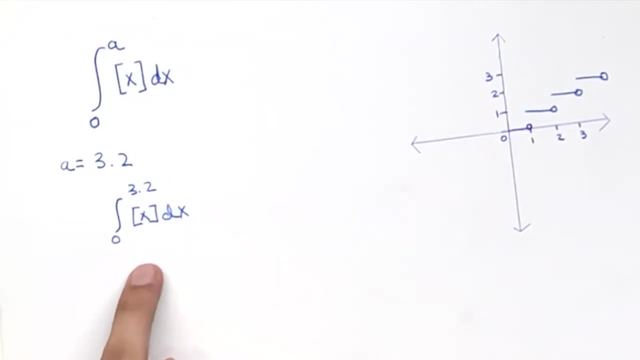 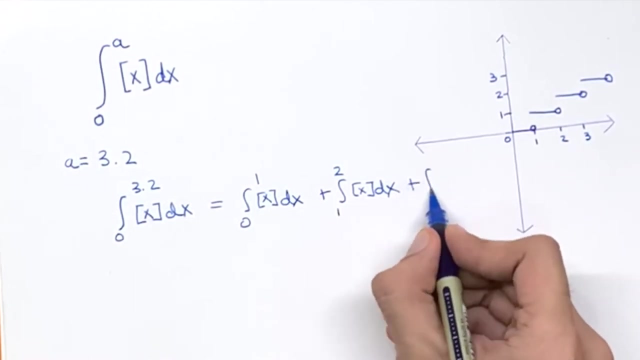 function of x, dx. This can be written as the integral from 0 to 1 of the greatest integer function, plus the integral from 1 to 2 of the greatest integer function, plus the integral from 2 to 3 of the greatest integer function. And now we have to take the integral from 3 to 3.2.. 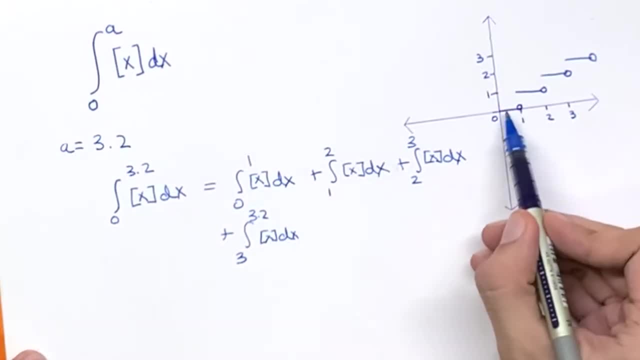 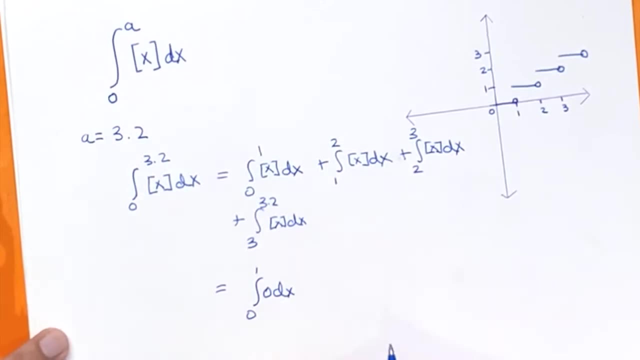 So, from 0 to 1, the value of the greatest integer function is just 0. So we can replace that with the integral from 0 to 1, 0 dx. We are replacing this with a 0 because from 0 to 1, the value of this is a constant, So we will. 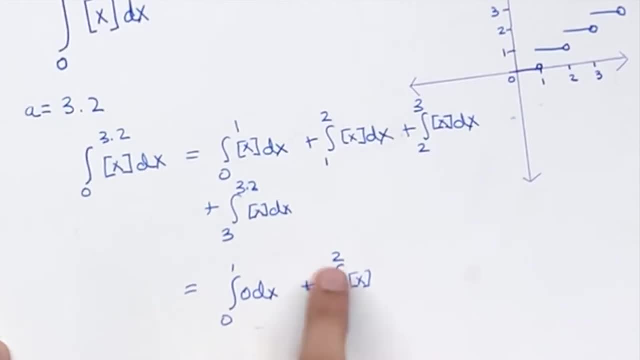 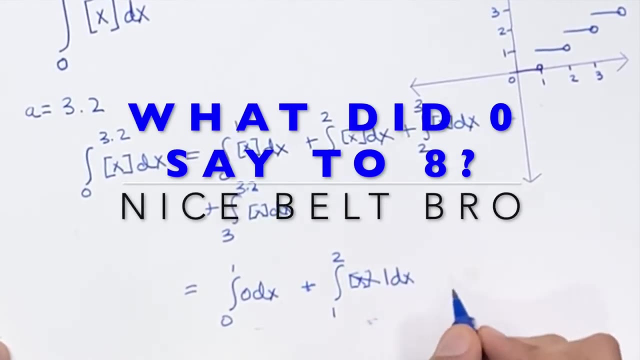 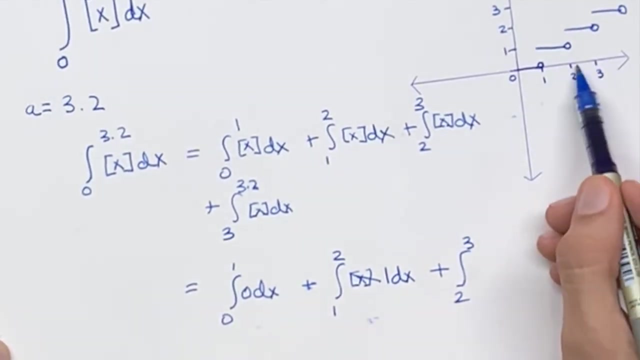 treat it like a constant. Similarly, from 1 to 2, the greatest integer function, x, has the value of 1.. So we can replace this with 1 dx. From 2 to 3, the greatest integer function has the value 2.. 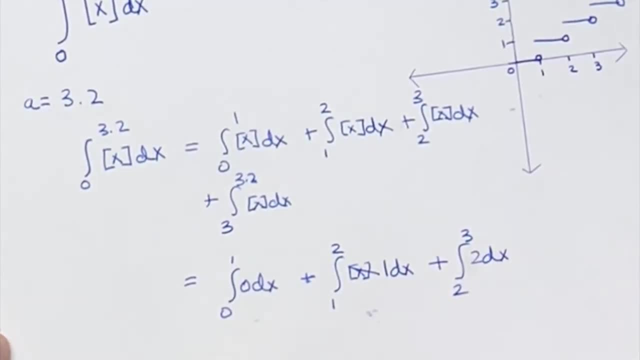 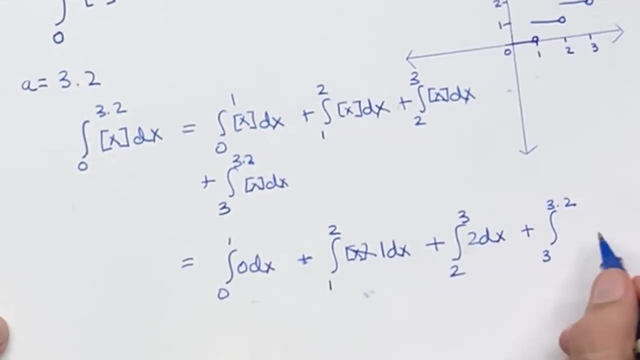 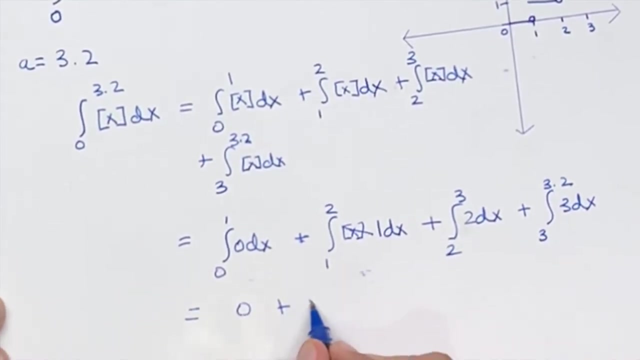 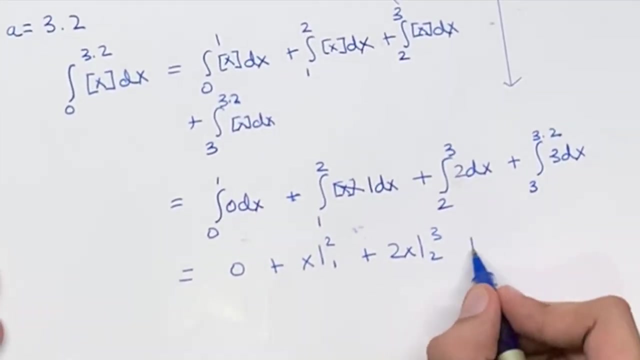 So we replace a 2dx here, and for the final one we can put the value 3dx. So this gives us 0 plus x from 2 to 1 plus 2x from 2 to 3 plus 3x from 3 to 3.2.. So let's. 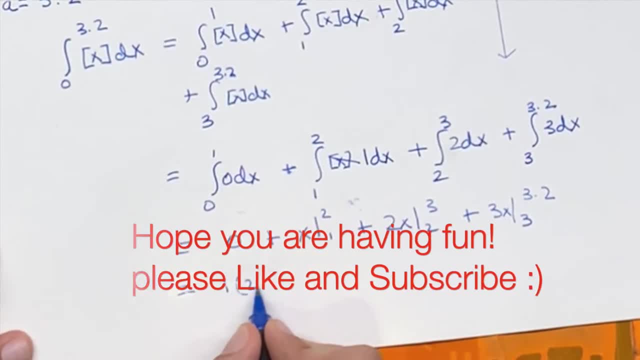 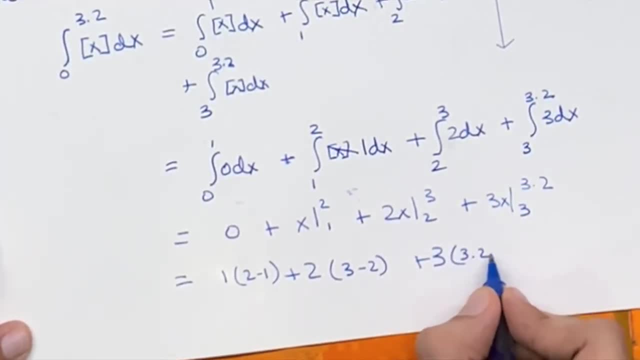 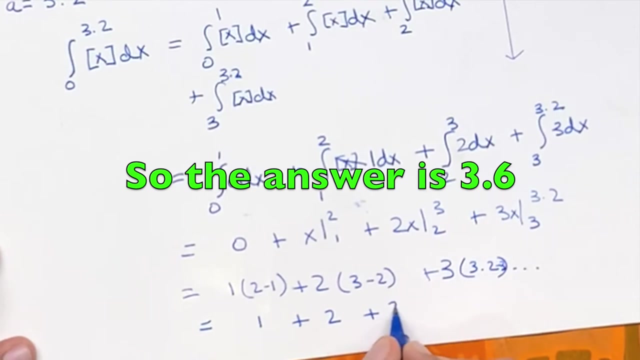 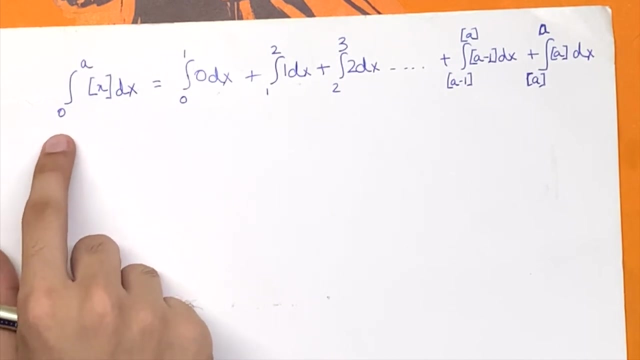 evaluate this. This gives us 1 times 2 minus 1 plus 2 times 3 minus 2 plus 3 times 3.2 minus 3.. So now let's look at the generalized answer of the integral from 0 to a of. 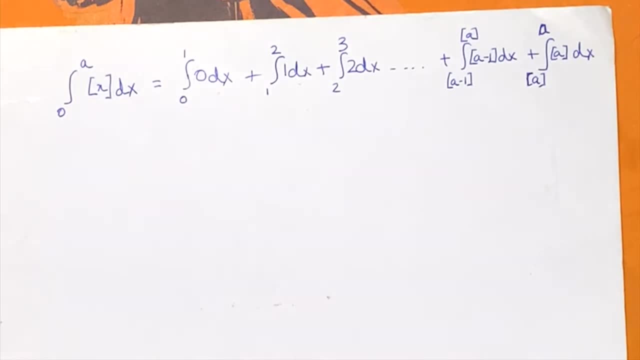 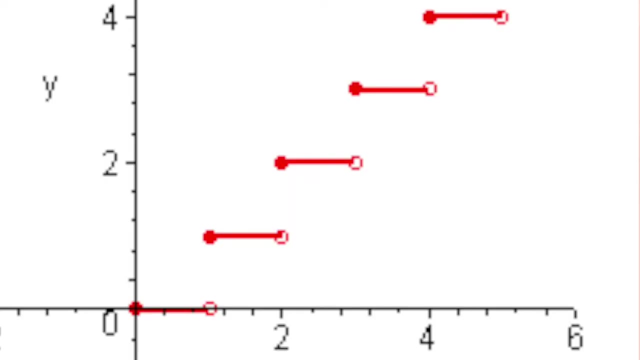 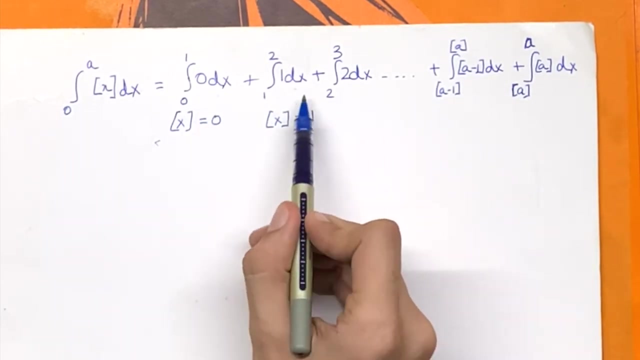 the greatest integer function of xdx. We can rewrite this integral as a sum of numerous other integrals. So, from 0 to 1, the greatest integer value function of x will give us 0. So we can write this as a constant. Similarly, the value here will be 1 and so on. So this will give us 0. 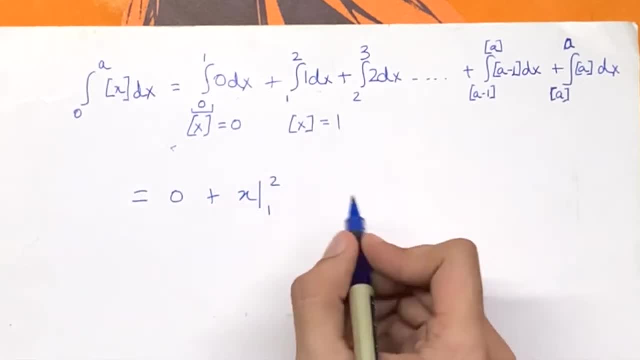 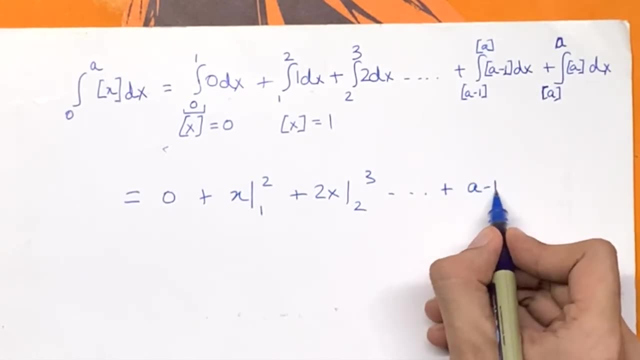 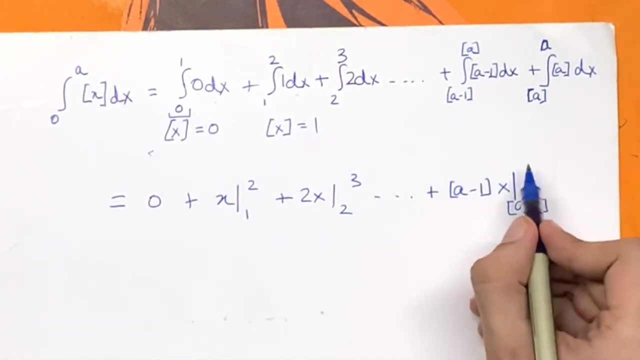 plus x from 1 to 2 plus 2x from 2 to 3, and so on, up to the greatest integer value of a minus 1 x. from the greatest integer value of a minus 1 to the greatest integer value of a. 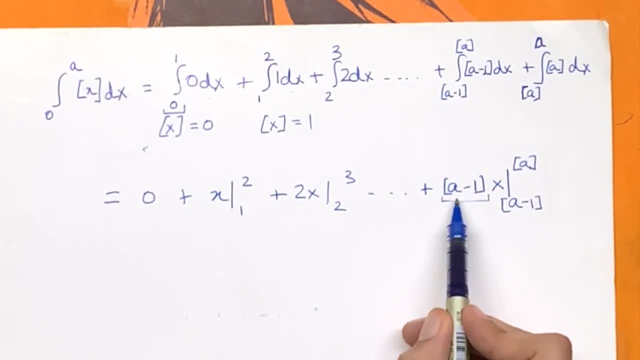 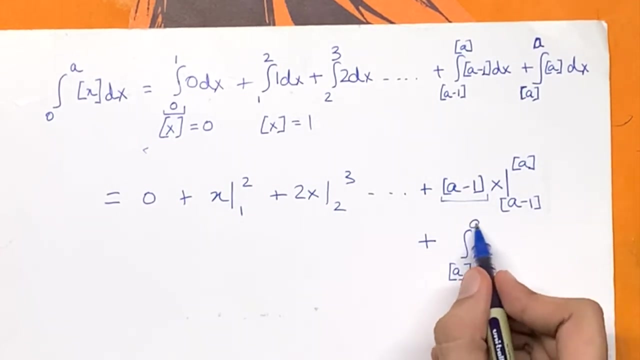 So in the previous example we put 2 here because a was 3.2 and the greatest integer function of a minus 2 would have given us 2 from 2 to 3, and now we have to add that last extra part from the greatest integer function, a to a In. 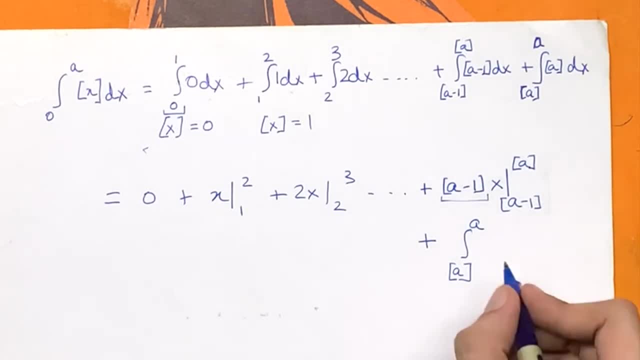 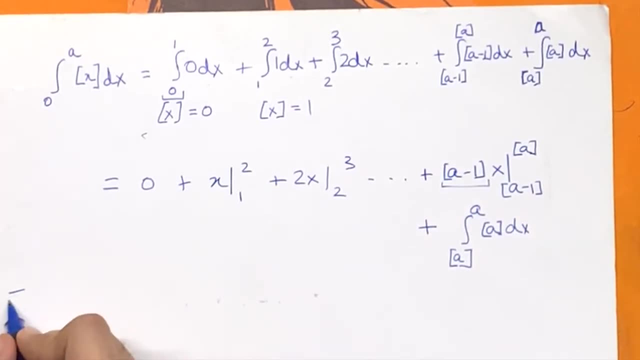 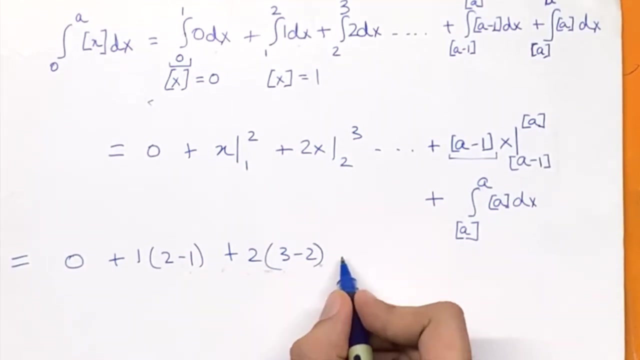 the last example. this was from 3 to 3.2.. lower boundary, which is the greatest integer value of a dx. So this gives us 0 plus 1 times 2 minus 1 plus 2 times 3 minus 2. all the way up to 1 minus a, all the way up to the greatest integer. 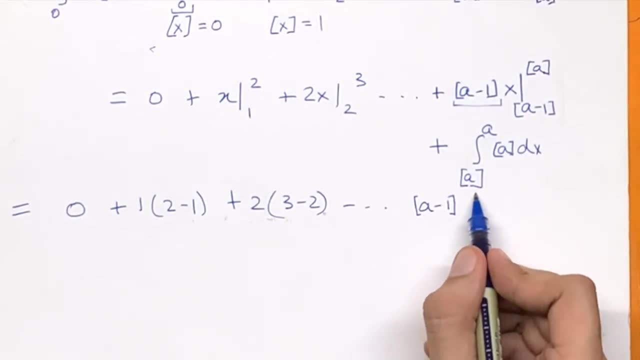 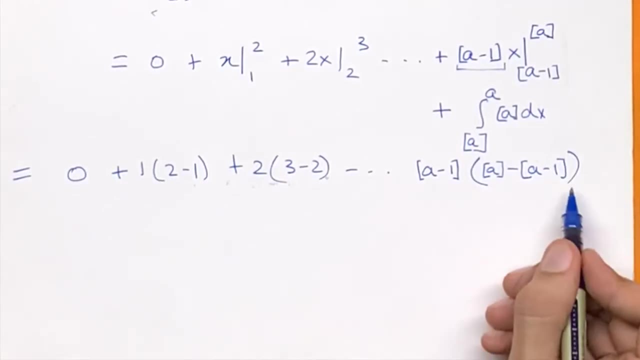 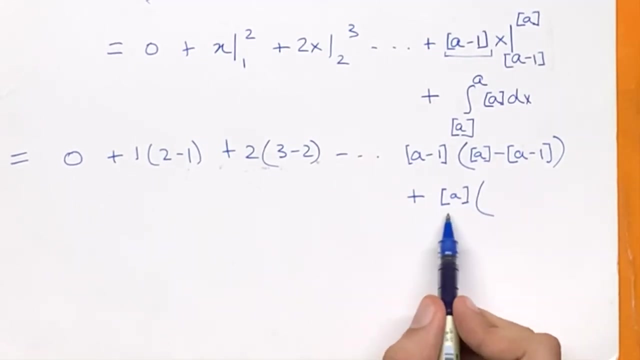 function of a minus 1, multiplied by the greatest integer function of a minus the greatest integer function of a minus 1.. This will just become 1 plus the greatest integer function from a plus the greatest integer function of a times a minus the greatest integer function. 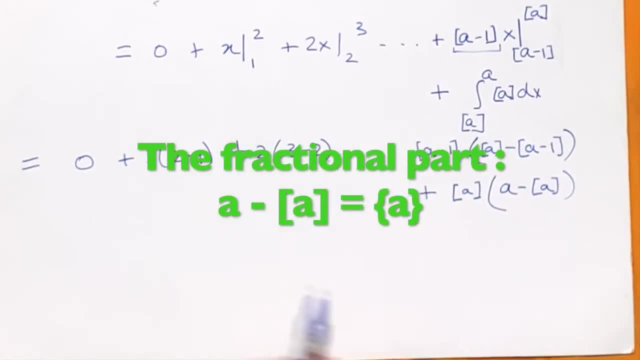 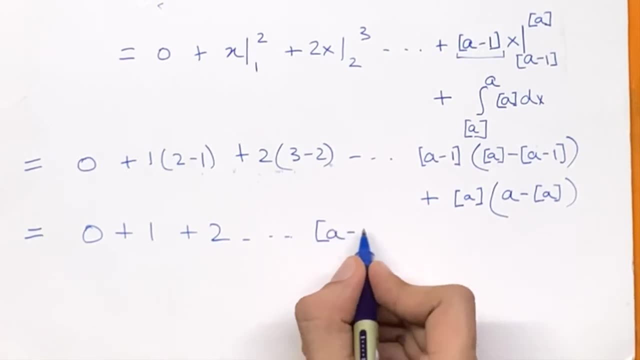 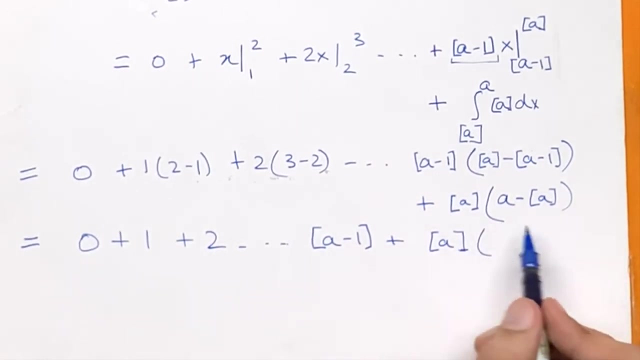 of a. So this is just the last decimal part. So we have 0 plus 1 plus 2, all the way up to the greatest integer function of a minus 1 plus the greatest integer function, a plus, multiplied by the decimal part of a, that is, a minus. the greatest integer function of: 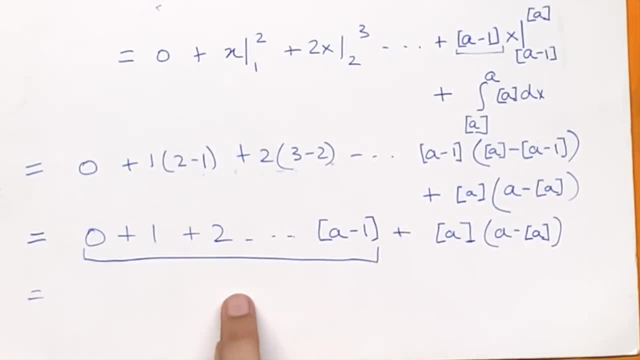 a. So we can write this as the sum of all the numbers up to the greatest integer value of a minus 1.. So that will be the greatest integer value of a minus 1 times the greatest integer value of a minus 1 plus 1 upon 2, plus the greatest integer value of a times the.